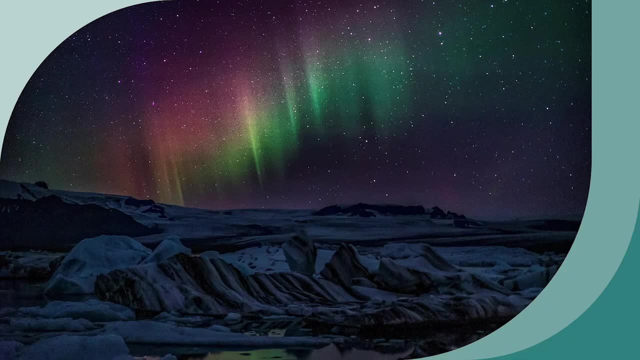 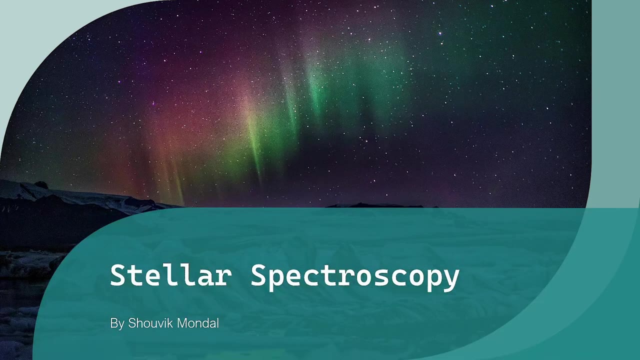 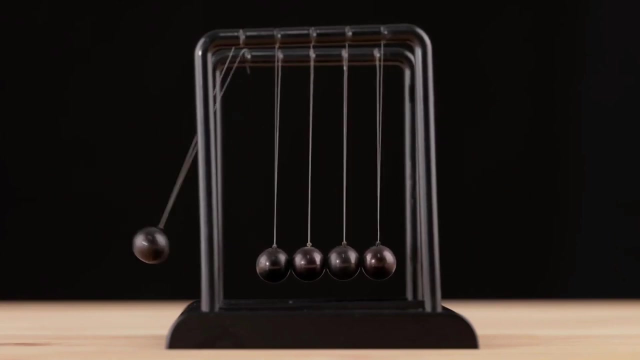 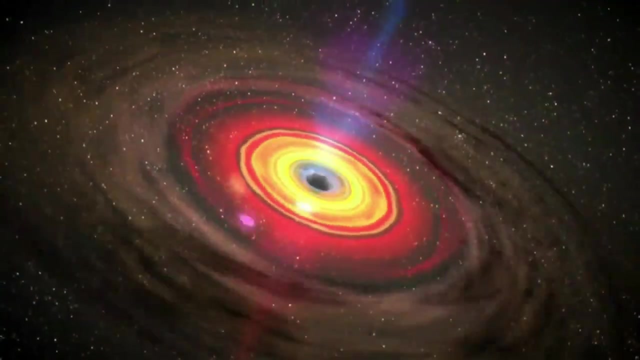 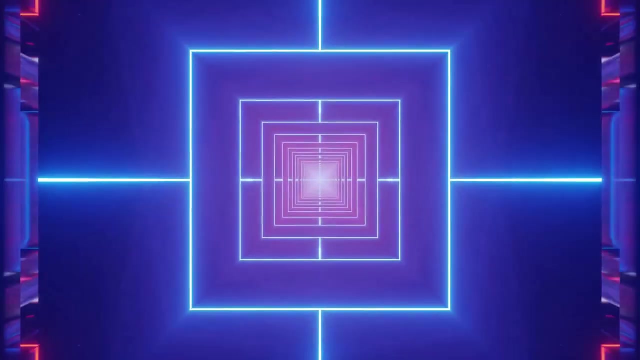 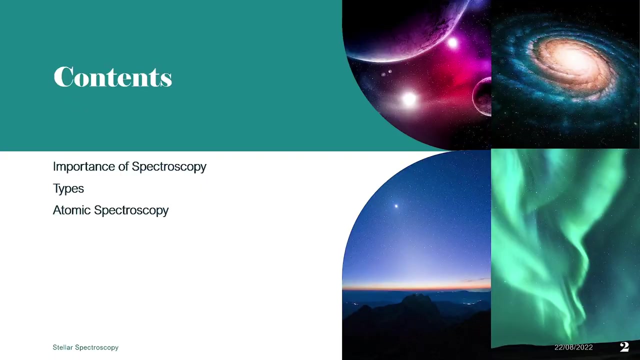 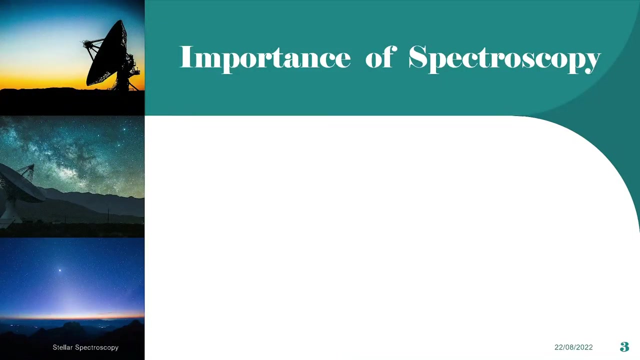 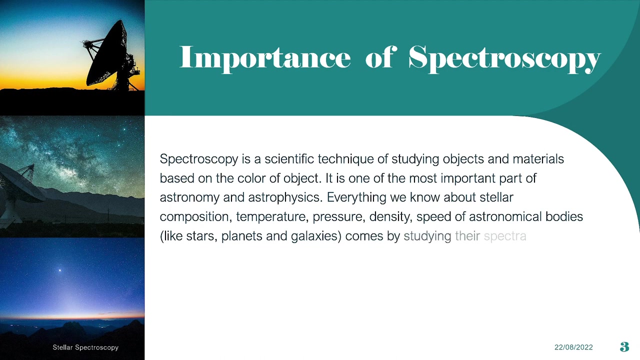 Hello everyone, this is Shouvik and you are watching College Level Physics. Today, I am going to talk about some basic and important aspects of stellar spectroscopy. So let's get started. The contents which I will be covering today are listed here, as you can see. Now come to the importance of spectroscopy. Now, spectroscopy is a scientific technique of studying objects and materials based on the color of object. It is one of the most important part of astronomy and astrophysics. Everything we know about stellar composition, temporary composition. 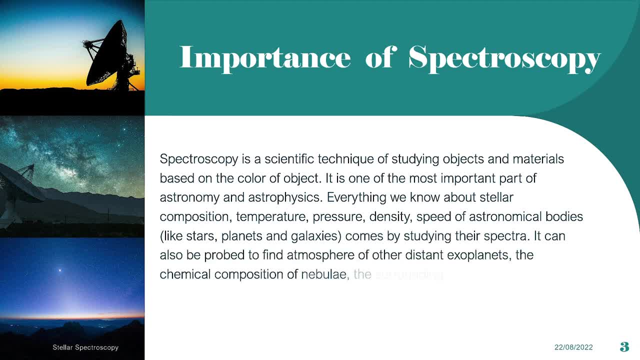 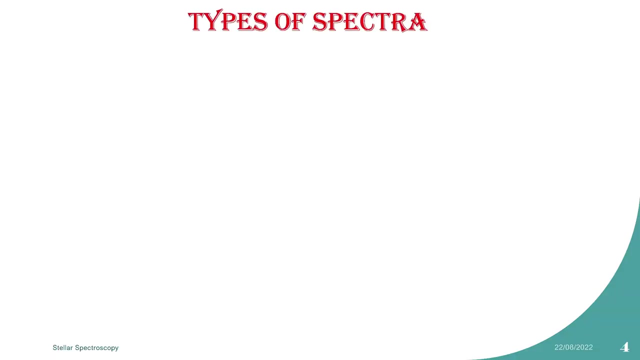 temperature, pressure, density, speed of astronomical bodies like stars, planets and galaxies comes. by studying their spectra, It can also be probed to find atmosphere of other distant exoplanets, the chemical composition of nebulae and the surrounding atmosphere of black holes, and many more. So let's move on to our next slide, which is the types of spectra. There are mainly three distinct types of spectra: Continuous spectrum, absorption spectrum and emission spectrum. 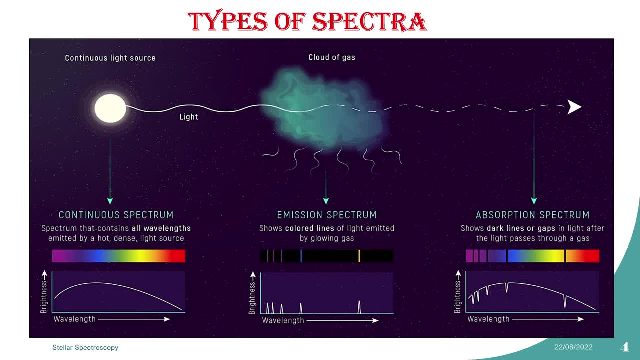 The continuous spectrum contains all wavelengths emitted by hot, dense light source, As you can see here. wait for a minute. I am choosing the laser point, As you can see in the first graph, this is the brightness versus wavelength graph of the light emitted by the source which is here is the star, And this is the continuous spectrum. as you can see, No dips or peaks are present here in this graph spectrum. And the second one is the emission spectrum, which shows the colored light. 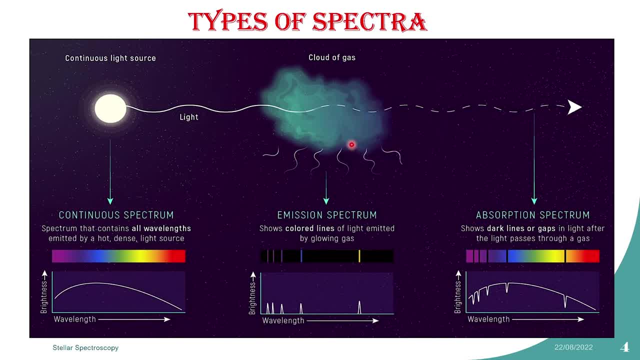 Here you can see the two lines of light emitted by the glowing gas, which is the cloud of gas And, as you can see, these are the peaks which are emitted by the minerals or elements present in this cloud of gas. And the third one is the absorption spectrum, which shows the dark lines or gaps in light after light passes through this cloud of gas. 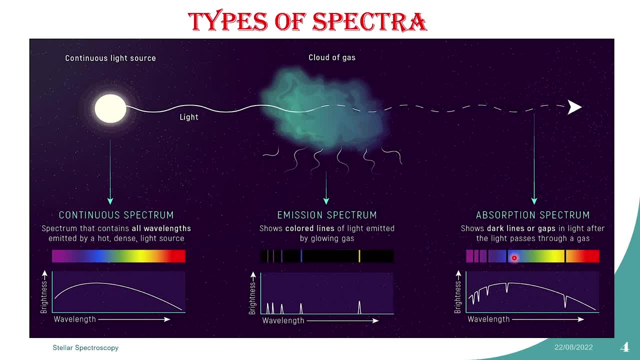 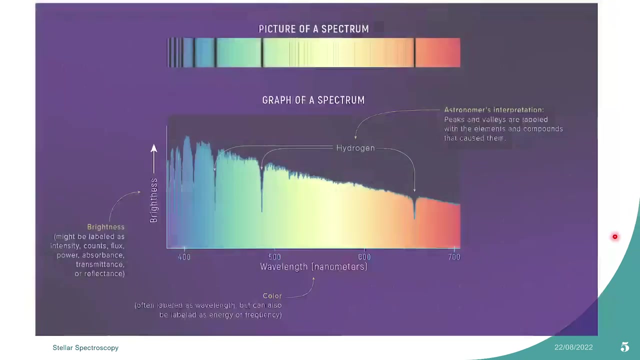 And you can see the pattern, or these values are present in the continuous spectrum, which are the signature of the different elements present in this cloud of gas which absorbs the light emitted by this star and then, when it emits, we get the emission spectrum. So now let's move on to our next slide. As you can see, this is an artistic illustration. 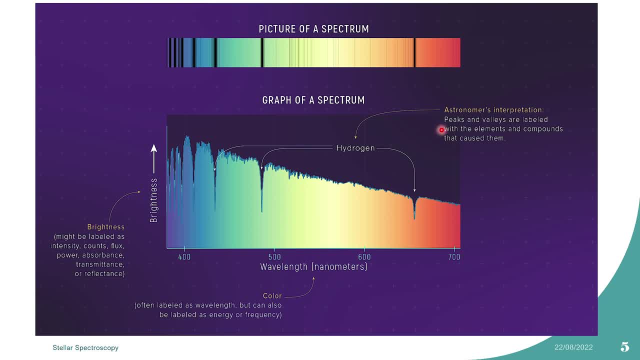 of a picture of a spectrum. This is not a real one, but, anyhow, these dips are due to the hydrogen atoms and, as you can see here, this is also the brightness versus wavelength curve, and the peaks and valleys are level with the elements and compounds that cause them. and, as I have said, 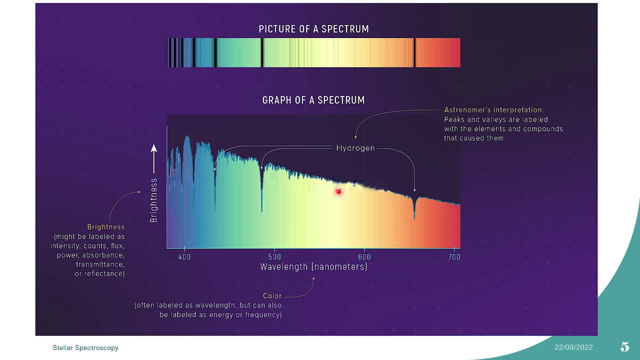 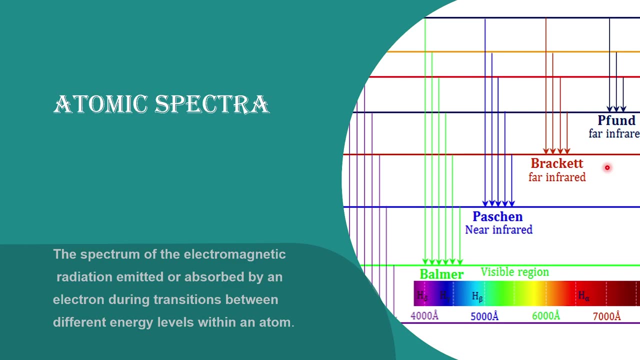 earlier that this is due to the hydrogen atom's presence in the stars or the cloud of gas. Now these spectra are mainly produced by atoms and molecules. So now let's move on to our next topic, which is the atomic spectrum. Now, in atom, the transition occurs mainly due to the electronic jump in different energy levels. 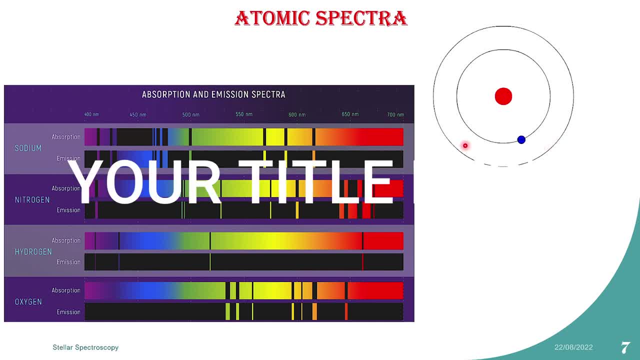 Imagine Bohr's atomic model like this one. when the atom jumps from this level to this level, it emits some radiation, which we call light. actually, if it's fall on the visible spectrum, we see it. if it doesn't, we don't see it from our eyes. actually, we observe it in different instruments. 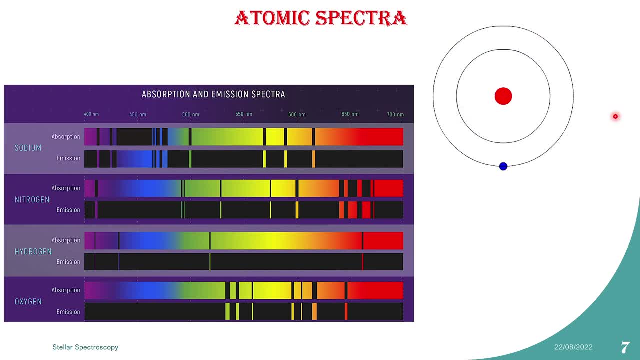 but anyhow. so we can see distinct line spectrum in each atom. but for molecule it's difference, as we will see later. but here this is the absorption spectrum of sodium atom and this is the emission spectrum. as you can see, these two are the complementary to each other and the second one is the due to. 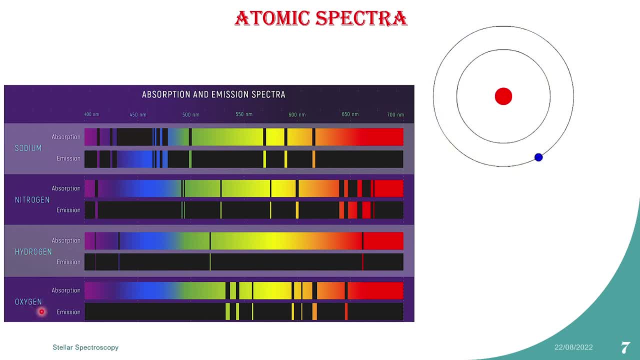 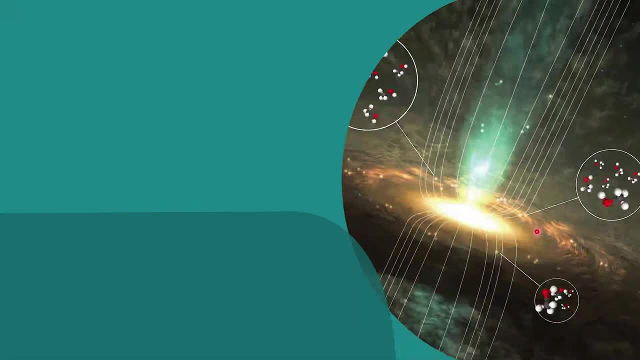 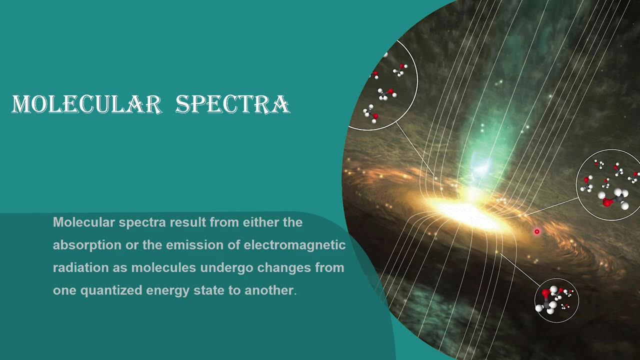 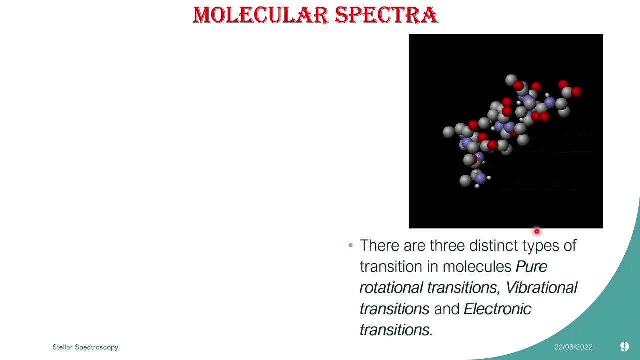 nitrogen atom, the third one is hydrogen and the fourth one is oxygens. so let's move on to the next slide, Which is the molecular spectra. now there are three distinct types of transition molecules: pure rotational transitions, vibrational transitions and electronic transitions. now this is a schematic diagram showing how the transition 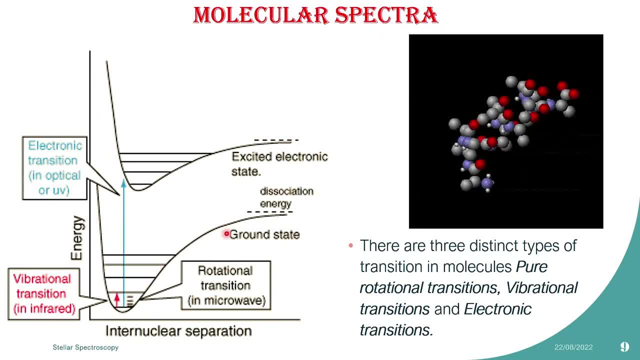 occurs now. these two curves are called the Morse potential, and when electron jumps from this curve to this curve, it is called the electron transitions and it falls in the optical or ultraviolet regime of electromagnetic radiation. and this horizontal lines are due to the vibrational motion of the 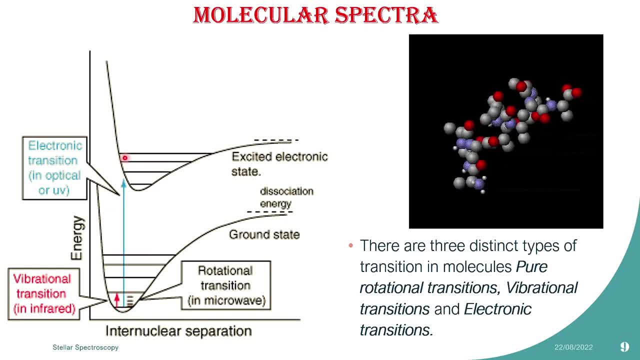 molecule and when transition occurs between these two levels, we call it a vibrational transition, which it falls in the infrared regime. and this tiny horizontal lines, as you can see here I am pointing this is due to the rotational motion of the molecules when the transitions occur between different 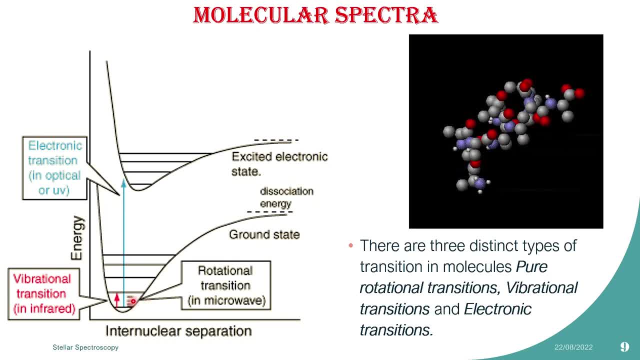 levels of this- rotational motions or the rotational spectrum, call it the rotational transitions, and which falls in the microwave regime. so- and this is a GIF of a particular element I can't recall now, and here you can see this- atoms are jiggling and vibrating and also having some rotation. but 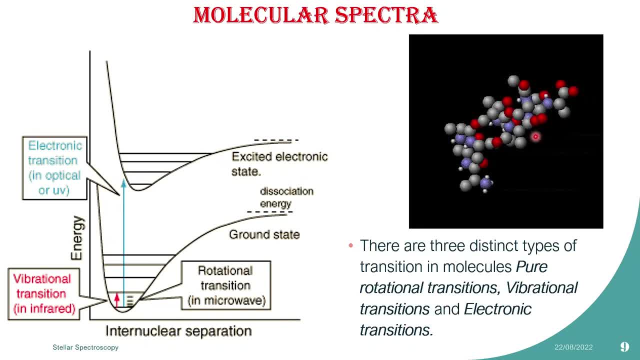 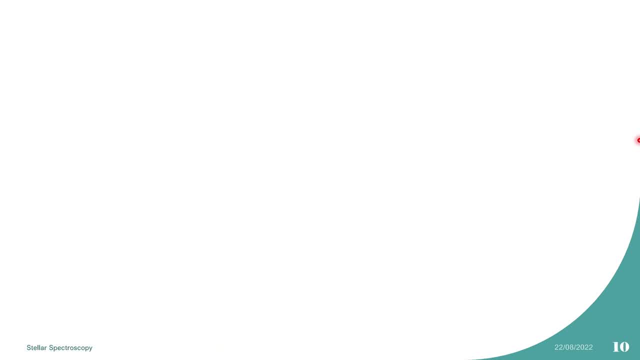 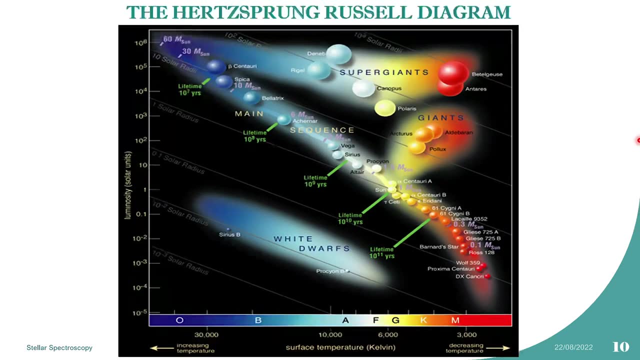 you can see here the electronic jump, but anyhow, this is a beautiful illustration, as I have found on the internet. so move on to the next topic, which is the HR diagram or the Hirschsprung-Russell diagram. this is the famous Hirschsprung-Russell diagram, which is a plot of 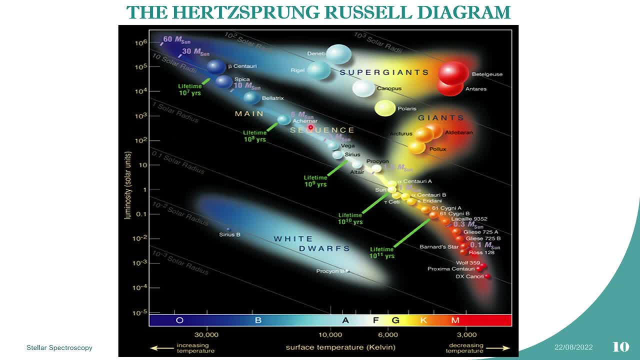 temperature versus luminosity of stars. now, depending on its initial mass, every star goes through specific evolutionary stages, dictated by its internal structure and how it produces energy. each of the stages corresponds to a change in the temperature and luminosity of star, which can be seen to move to. 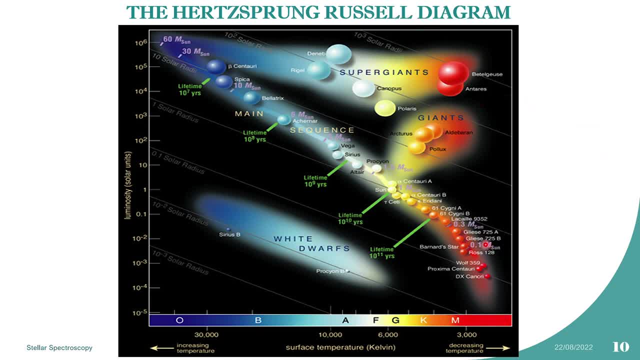 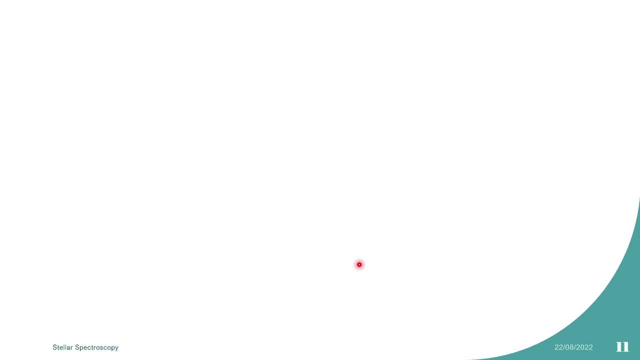 different regions on the HR diagram as it evolves. this reveals it here in the HR diagram. astronomers can know a star's internal structure and evolutionary state simply by determining its position in the diagram. so now move on to our next topic, which is the stellar spectral classification. how do we classify the spectrum of different 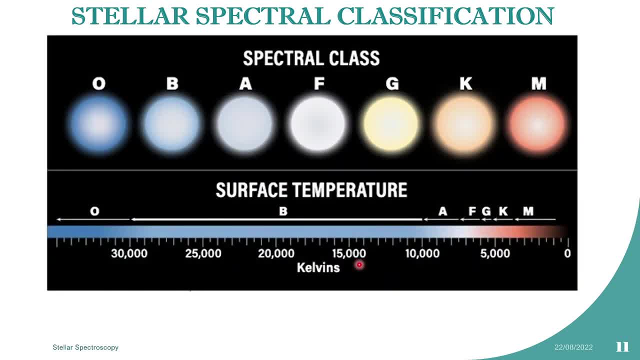 stars. now we can classify different types of stars based on their surface temperature. now there is a famous mnemonic stating that O be a fine-gird gizmi, where O denotes the hottest temperature star and, as we go along, where M denotes the coolest star and, for example, our Sun is a G to B type star and 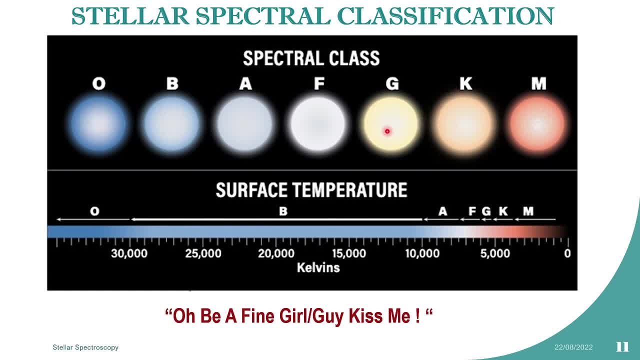 which falls in around in this region in between G and middle of the gate. so this is how you can remember the temperature of star: where O is the hottest and M is the coolest, it gradually decreases from O to M. so now move on to the next topic. 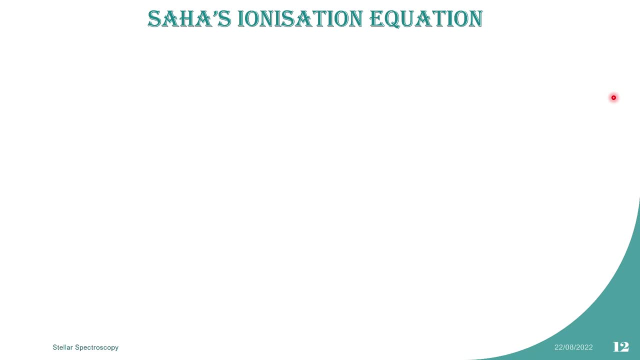 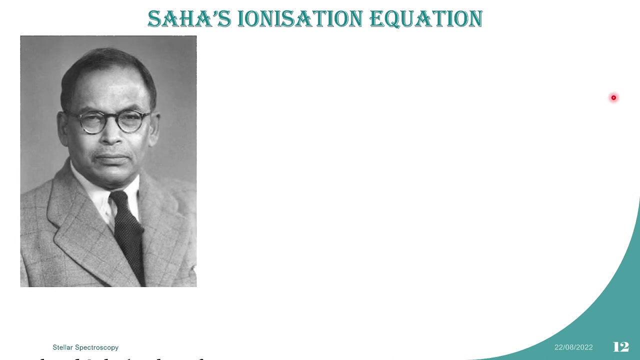 which is Saha's ionization. now, if I don't include this topic- Saha's ionization question, this presentation would be incomplete, as we all know that Magna Saha was the first scientist to give a proper explanation of what causes the spectral lines of stars, for which we call him the father of stellar spectroscopy. 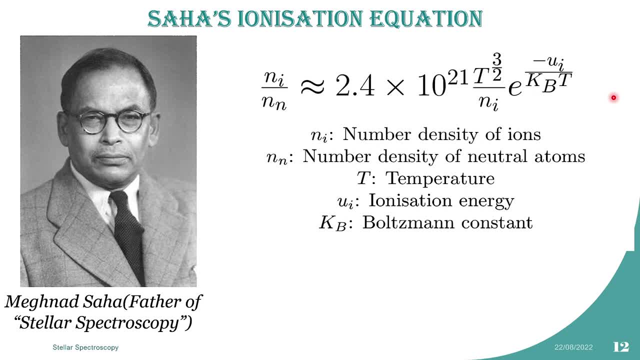 now, this is the famous Saha's ionization equation, actually, where I have put the values of the different constants and get this particular value, and here I have written down this particular variables, where so now is the number of the number density of ions, and N is the number density of neutral atoms and T is the 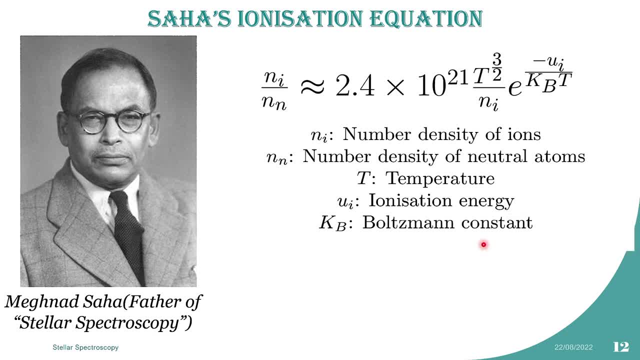 temperature, Ui is the ionization energy and Kb is the Boltzmann constant. if you put this value, depending on which stars you are looking at, you will get the number, density of ions present in those stars, the abundance of different elements present in the star actually. so, finally, 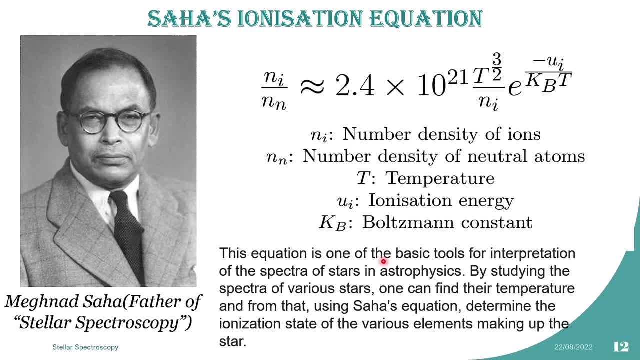 this equation is one of the basic rules for interpretation of spectra of stars. by studying the spectra of various stars, one can find their temperature and from that, using Saha's ionization question, determine the ionization state of various elements making up the star. as I had said earlier, 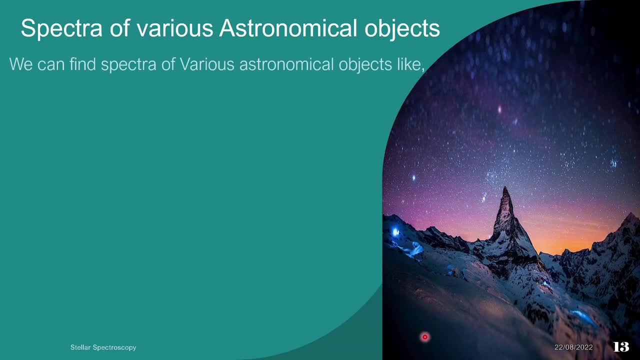 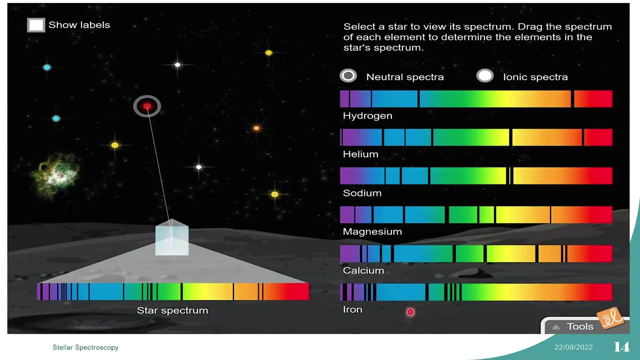 so you can find spectra of various astronomical objects like stars, galaxies, Nebula, exoplanets, black holes, questions and any such objects, and we will see some of them. like if you probe into a star surface, you might get this type of spectral image, but it varies from start to start depending on what kind of star you are. 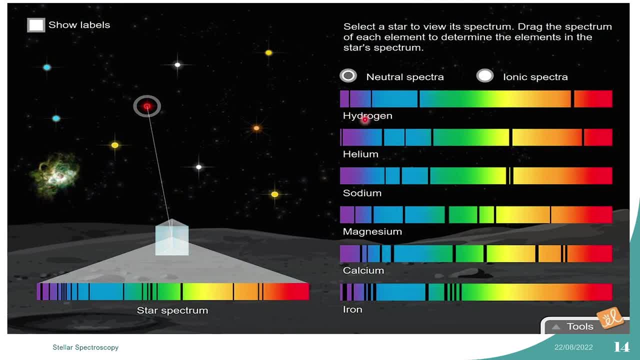 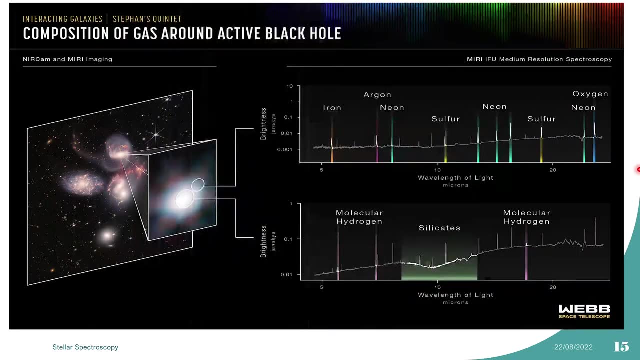 probing in what kind of elements are present in those stars and if it's hydrogen present, you will see this types of central and if helium this type of, and so on and so forth. so now this is the schematic picture taken by the jwst, which is the composition of 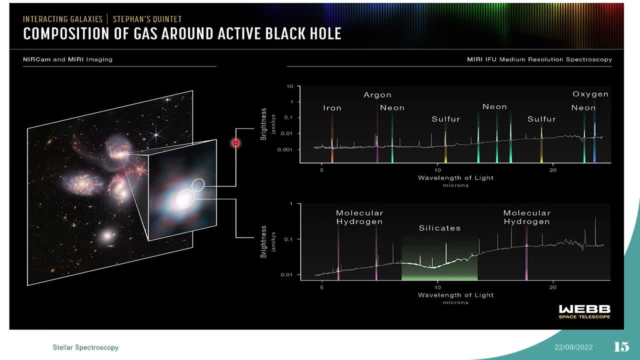 gas around active black hole in the internal interacting galaxy called stephen squintant. here you can see different types of elements present in the accretion disk of the black hole, which is nothing but a star falling on and pressing to this black hole, and you can probe. 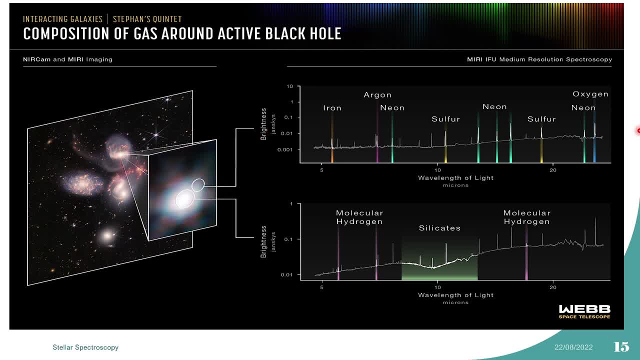 the surrounding atmosphere where you will get this different, this kind of spectrum, from where you can find the presence of argon, iron, neon, sulfur, oxygen and many such elements. and here you can see the molecular hydrogen silicates are also present in this particular surrounding of the black hole. so now move on to the next slide, which 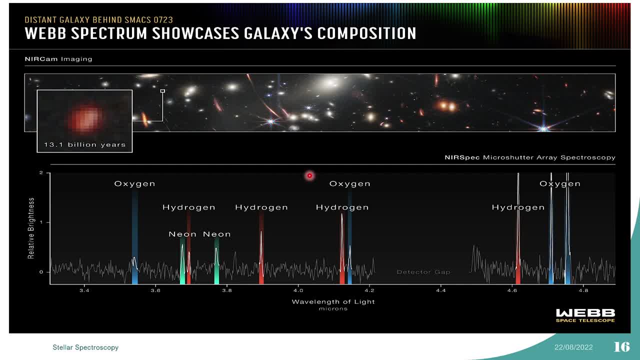 is the shows the chemical composition of a distant galaxy behind smacks 0.0723, which was captured by inaya cam of zwst. now, this galaxy was formed in the early universe, around 13.1 billion years ago actually, and if you probe into the details of this galaxy, you will find. 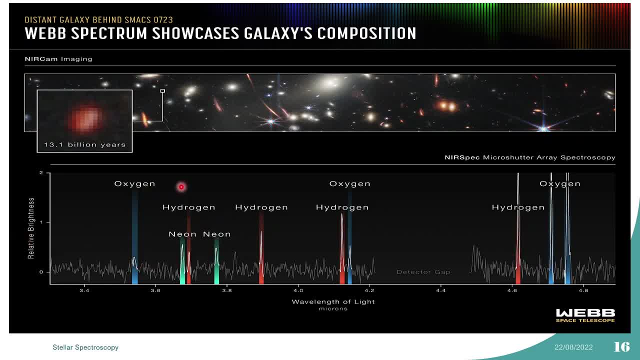 this kind of spectral image and where, from where you can get the information that oxygen hydrogen neurons are also present in this galaxy, found in this early universe? so this is the, but that's. the video that you will like to watch is very interesting. i hope you like these kind of the. subtitles and the chemical composition that we have printed out. you get a scan right here. so gas, neol, consig�, unglaublegibleesting galaxy gaia indicates one thing and there was a Naturally and Orbix Orth登онец. this doesn't mean you can see these particles autonomicつ. 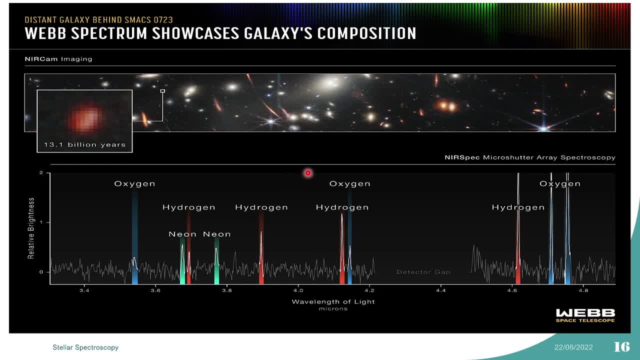 rockets that depend on the spectrum, that Sauce- I clicked into it- which could always affect the galaxies, how you can see the time university and the galaxy without study, which you can see here. so this is very exciting news, actually. now the next picture you are looking at is the atmospheric. 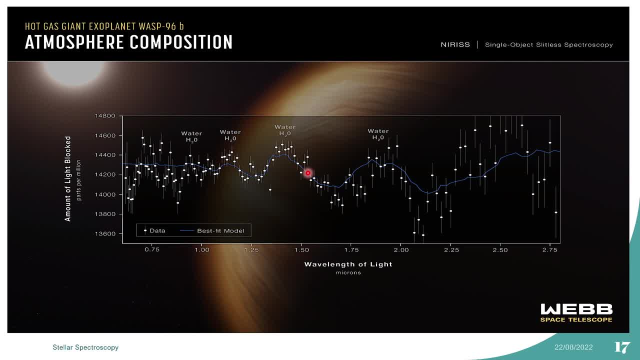 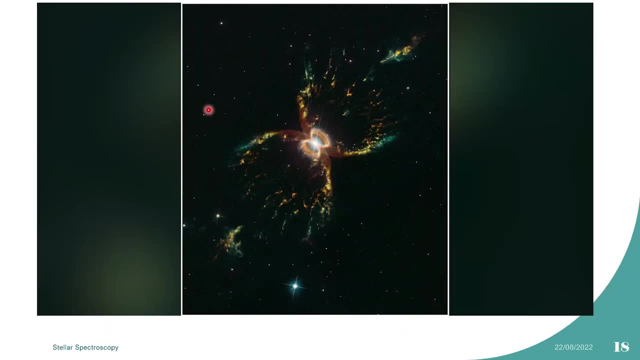 composition of hot gas, giant exoplanet called wasp 96b, where you can see the presence of water molecule, which is a very exciting news. actually, as you know, water is an essential component of life. so, finger crossed, what we found now? now, this is the spectroscopy of southern web, nebula and 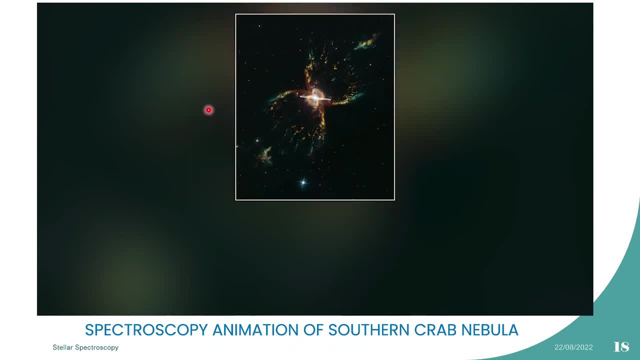 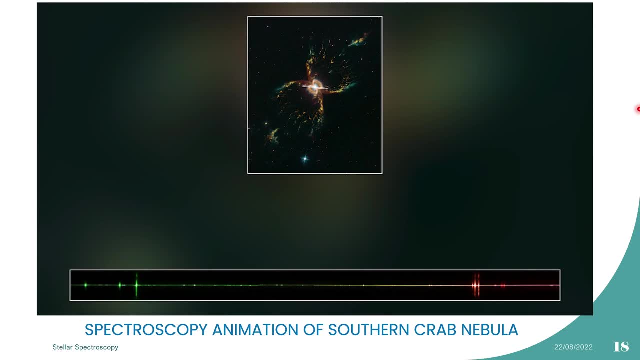 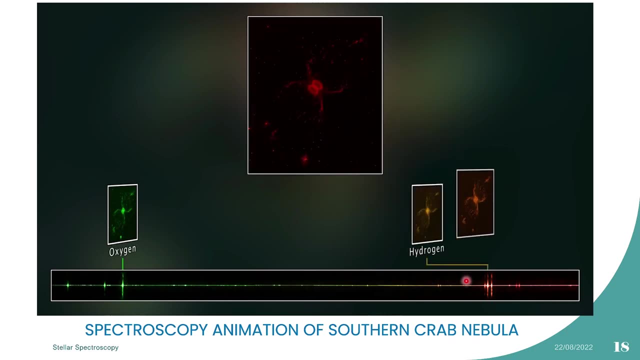 here. if you probe at the center of this nebula, you will find the spectral signature of different elements. for example, if you see here, this is the presence of oxygen, and this is due to hydrogen. next comes the nitrogen, and this is the oxygen, and this is due to hydrogen. next comes the nitrogen. 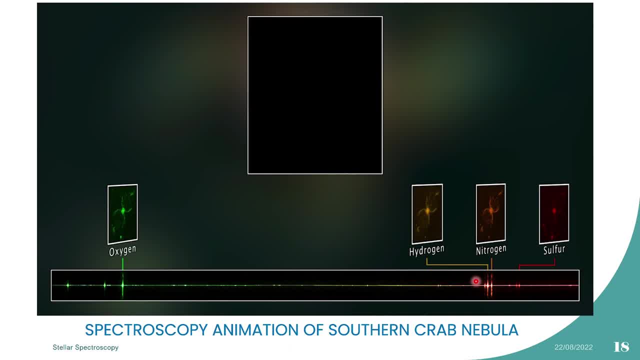 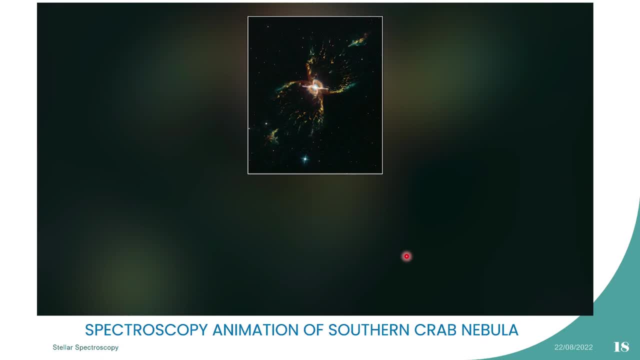 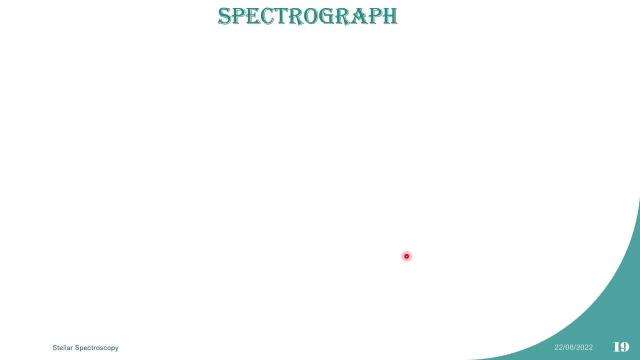 and this is due to oxygen and finally the sulfur. so if you use different kind filters, you will notice the presence of these kinds of elements. so next move on to our final pick up today's discussion, that is, the spectrograph. now, the spectrograph is an instrument used to obtain and record an astronomical spectrum. the spectrograph. 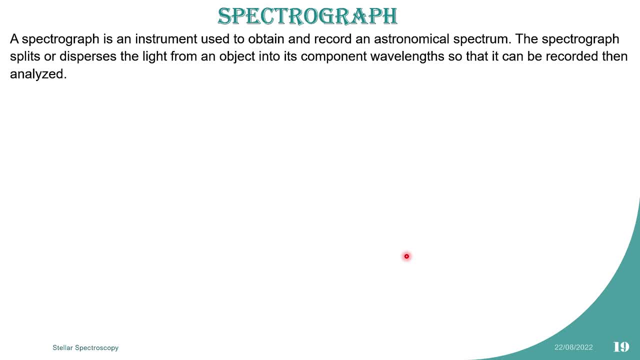 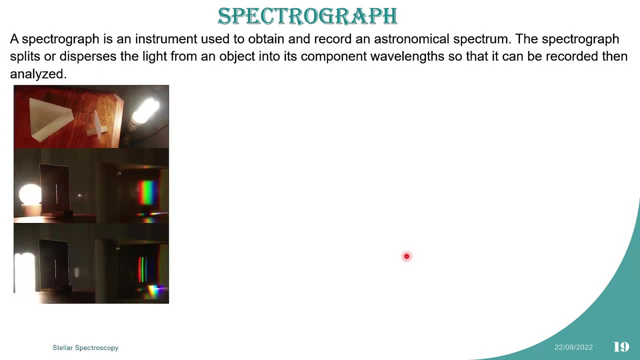 splits or disperses the light from an object into its component wavelength so that it can be recorded and then analyzed. now this is the most basic and simple of kind of spectrograph which uses only a prism. as you all know, this is a cfl lamp and this is actually an led lamp, where the prism splits. 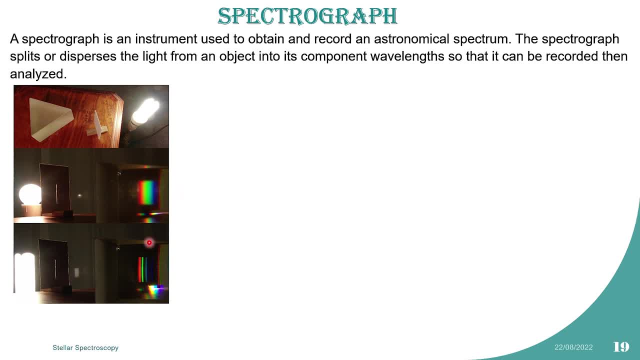 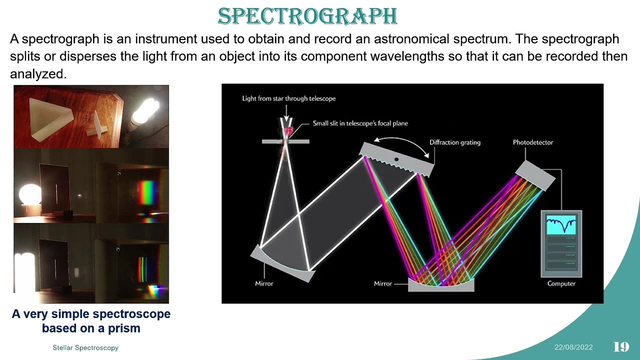 wavelength and you can see this pattern. you should actually try it at your home if you have one, this prism, so this is a bit advance spectrograph and this uses the diffraction grating and, as you can see, the light is falling through this slit into the mirror and this mirror focuses that light into this. 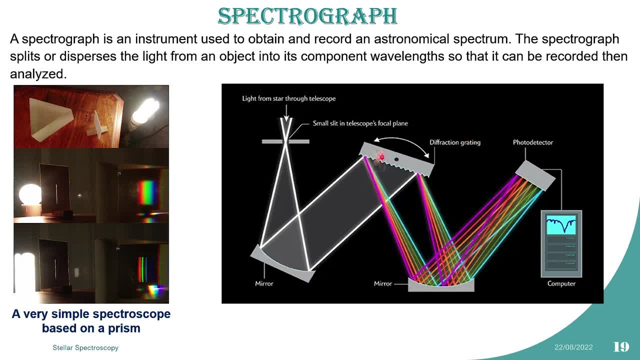 diffraction grating, where this diffraction grating actually splits the light into its multiple wavelength or component wavelength, and this mirror actually detects this light into the photo detector, through which it goes into the computer and then we analyze that light. so this is a bit advance spectrograph.